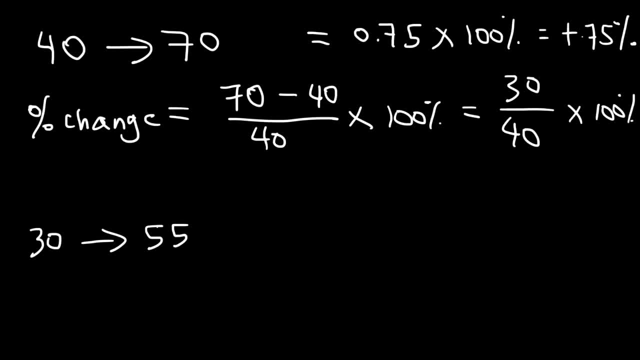 you positive 75%, so that represents a percent increase. so let's try the second example. the percent change is going to be the new value, which is 55 minus the original value of 30, divided by the original value times 100%. 55 minus 30 is 25, and so we have 25 divided by 30 now. 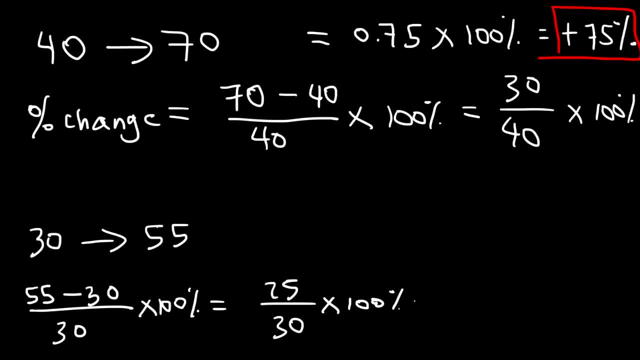 let's get the decimal value of that. so if you type in 25 divided by 30 in your calculator, you should get 0.83 repeated, and then multiply that by 100% and that should give you positive 83.3%, so that 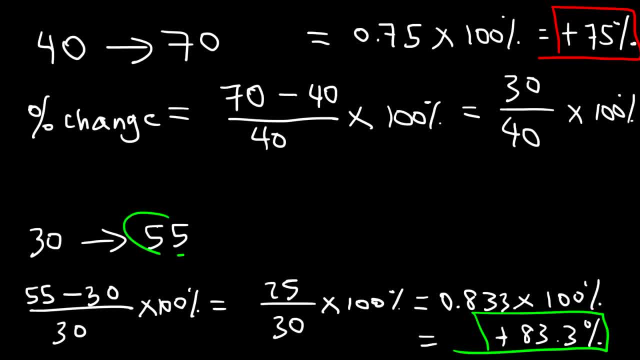 too, represents a percent increase. so anytime this number is larger than the first one, if the new value exceeds the original value, it will always be a percent increase. this number, your percent change, has to be positive. if it's negative, then it's percent decrease, and the only time you'll have that is if 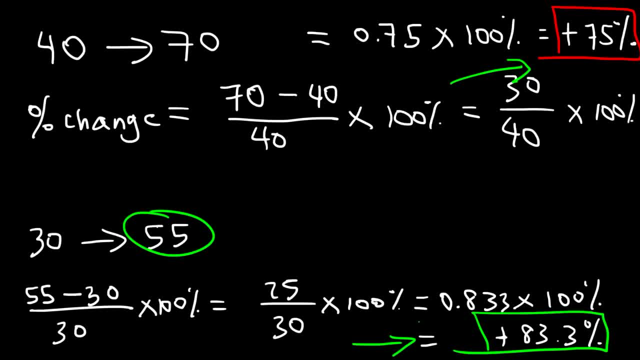 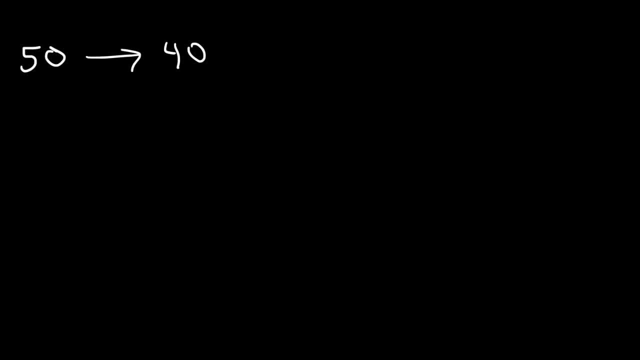 the new value is less than the original value. so let's say, if we have 50 decrease into 40, this is going to be a percent decrease because the new value is less than the original value. go ahead and calculate the percent change now. your answer has to be negative. the new value. 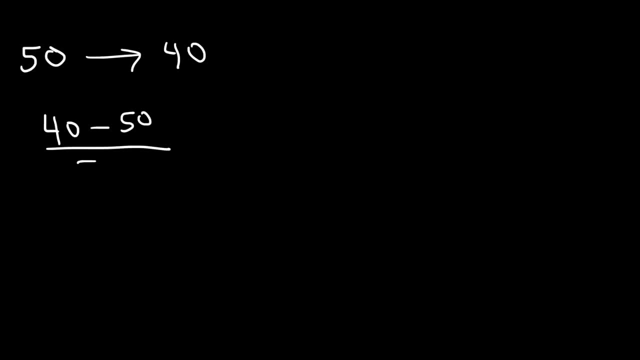 is 40, the original value is 50 and then we need to divide it by the original value and then multiply it by 100%. so 40 minus 50 is negative 10, negative 10 divided by 50. if we type that in, that's negative 0.2. so if you 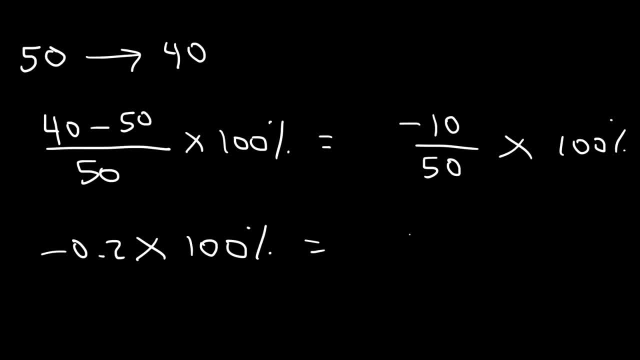 take negative 0.2 and then multiply it by 100%. you're going to get negative 20%, and so that represents a percent decrease. let's try some word problems. in 2017, the price of gas in a solar power plant in the United States is $1.5 billion. 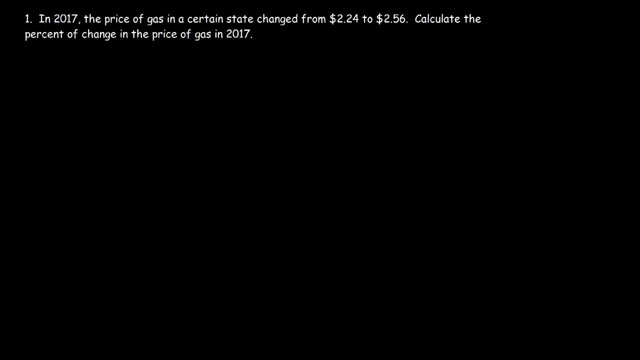 in 2017, the price of gas in a solar power plant in the United States is $1.5 billion. in 2017, the price of gas in a solar power plant in the United States is $1.5 billion. calculate the percent of change in the price of gas in 2017. so you need to. 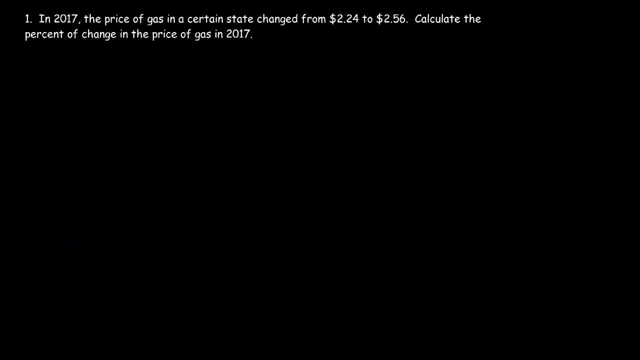 calculate the percent of change in the price of gas in 2017. so you need to value is 224. the new value is 2.56, so now we can calculate the percent change. It's going to be the new value, which is $2.56 minus the original value of $2.24, divided by the original times, 100%. 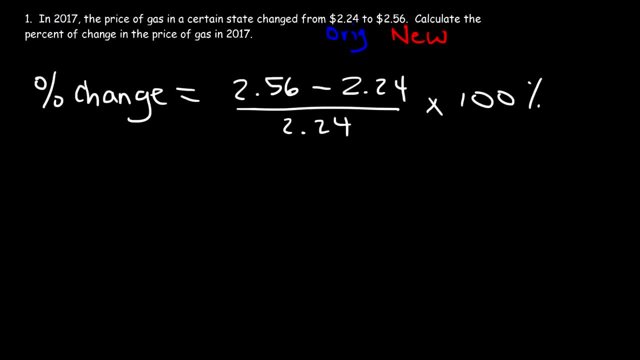 Now we're going to follow the same process. First we're going to subtract 2.56 by 2.24.. And you should get 0.32.. And then we're going to divide 0.32 by 2.24.. 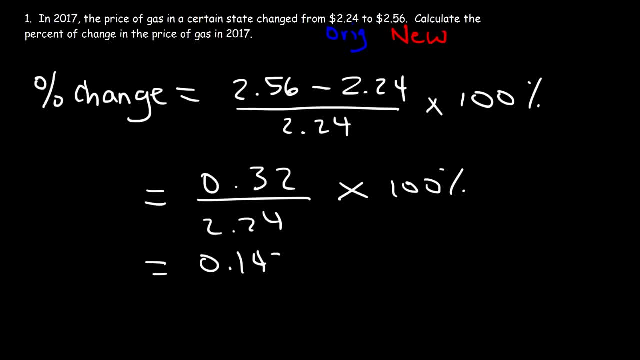 And that will give you 0.1429. if you decide to round it, Then multiply that by 100% And so this is going to be a percent increase And it's 14.29%. So that's the percent change. That's the 4% increase in the price of gas in 2017 in that state. 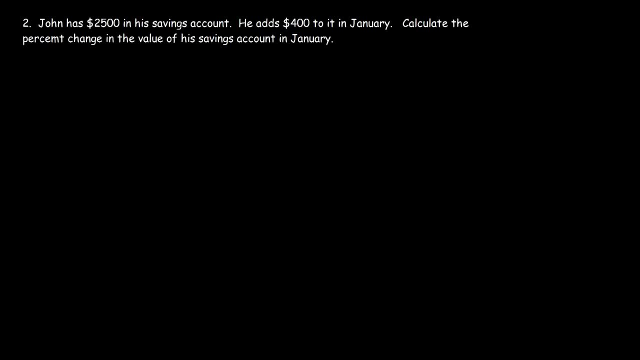 Number two: John has $2,500 in his savings account. He adds $400 to it in January. Calculate the percent change in the value of his savings account in January. So feel free to take a minute and work on that problem. So we need to identify the new value. 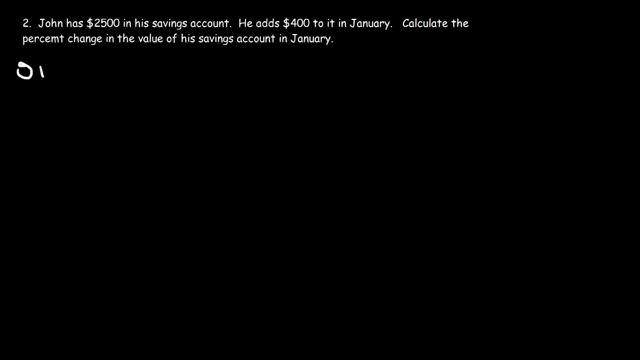 And the original value. So what is the original value in this problem? The original value is the money that he has in his savings account: It's $2,500.. Now what is the new value in his savings account? It's not $400.. 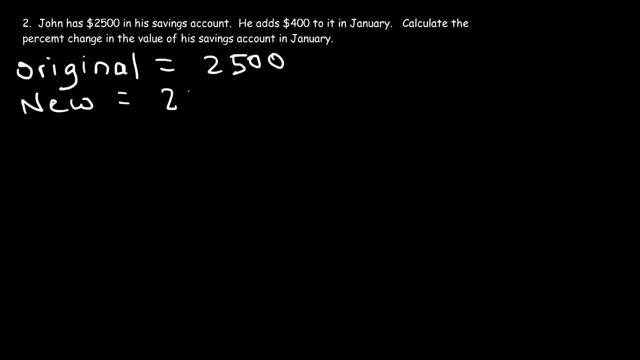 Remember he adds $400 to it. The new value is going to be $2,500 plus $400. Or basically $2,900.. The $400 is basically the change in the account in January. So now let's calculate the percent change. 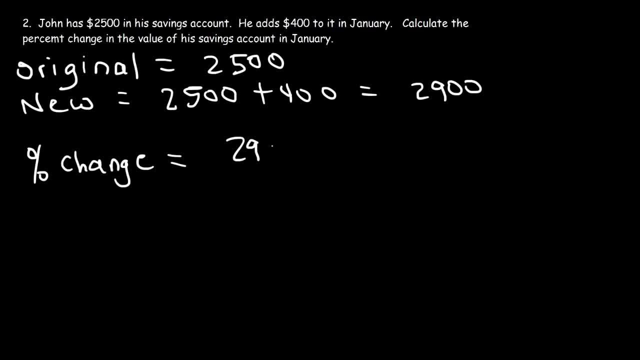 It's the new value of $2,900 minus the original value of $2,500. divided by the original value times 100%. So $2,900 minus $2,500, that's $400.. And let's divide $400 by $2,500.. 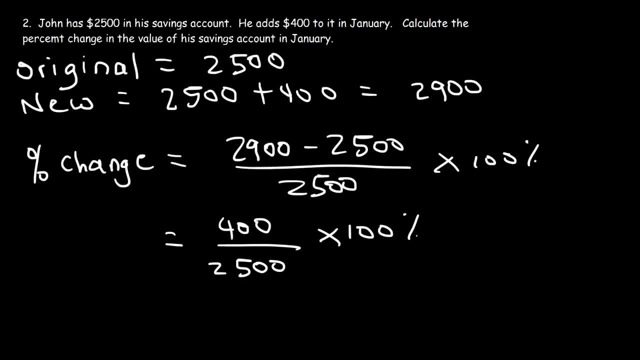 $400 divided by $2,500 is $0.16. And if you multiply $0.16 by 100%, you'll get 16%. So this is a percent increase. So his savings account went up by 16% during that month. 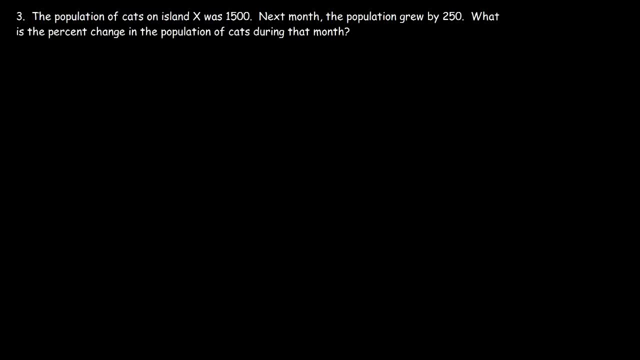 Here's another one. The population of cats on Island X was 1,500.. Next month the population grew by $2,500.. What is the percent change in the population of cats during that month? So first we need to identify the original value. 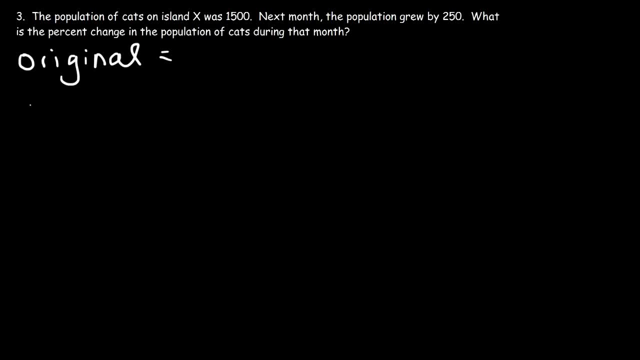 So what is the original value in this problem And also what is the new value? The original value is the 1,500 cats on a population. Now the population grew by $2,500.. So the new value is $1,500 plus $2,500. 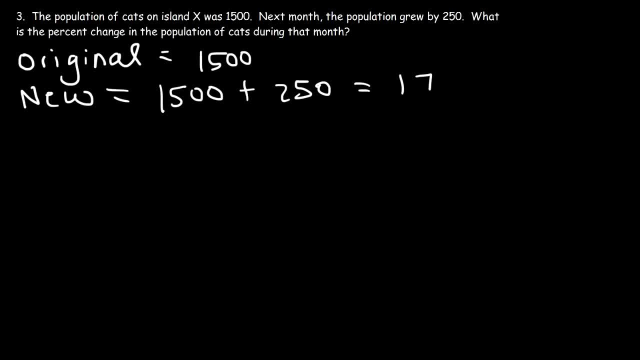 Which gives us a new value of $1,750.. So we need to use these two numbers in the formula. So now let's calculate the percent change. It's going to be the new value of $1,750 minus the original value of $1,500.. 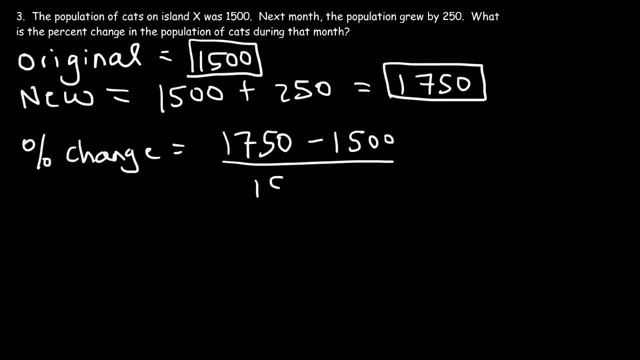 Which will equate to $250.. And then divide it by the original value, So $1,750 minus $1,500, that is the change. That's the $250 that we had at the beginning, And if we divide that by $1,500, that is going to give us, let's see, 0.16 repeating. 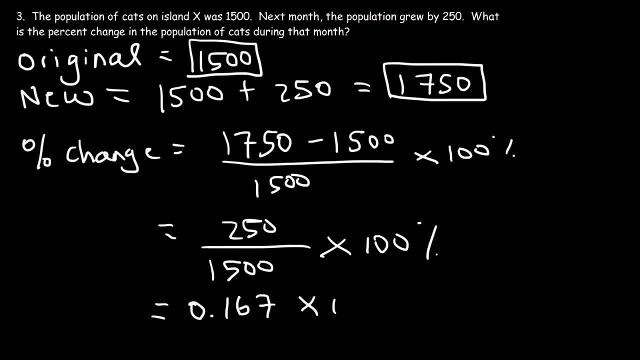 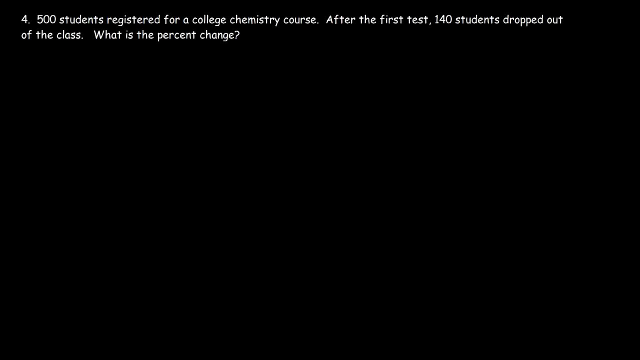 I'm going to round it to 0.167.. So this will give us a percent increase of 16.7%, And so that's the answer for this problem. Number four: 500 students registered for a college chemistry course. After the first test, 140 students dropped out of the class.